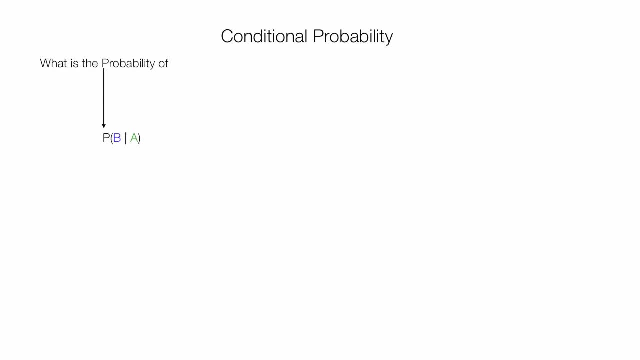 The P is. what is the probability That's the P And in this example, rolling a dice and its value is less than four is event B. Knowing that the value is an odd number, is event A. I could write it as this instead: What is the probability of rolling a dice and its value is less? 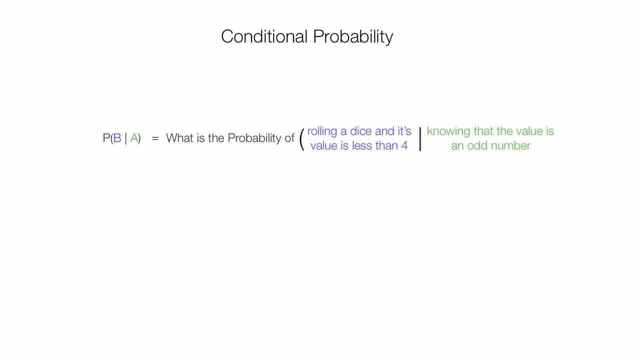 than four, And knowing that the value is an odd number. But that would be really cumbersome, and that's why statisticians use the shorthand notation that they do. So now the problem is all set up, and this is the equation We're going to find out. 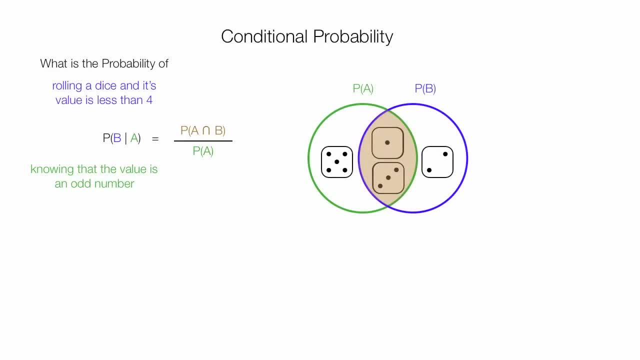 the values for this and I'm going to show you to use symbolically or visually as well. With a six-sided dice you could roll a one, a two, a three, a four, a five or a six. There is a one and six chance of rolling a one. 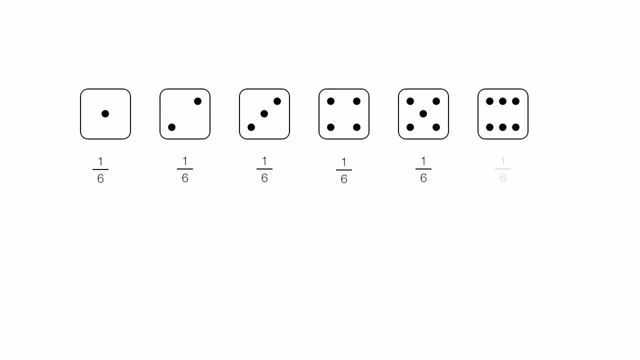 Or a three or a four or a five or a six, They're all the same. If I add all these up, if I actually add up all the ones, they equal to six. So I have six over six or one, which means everything's covered. 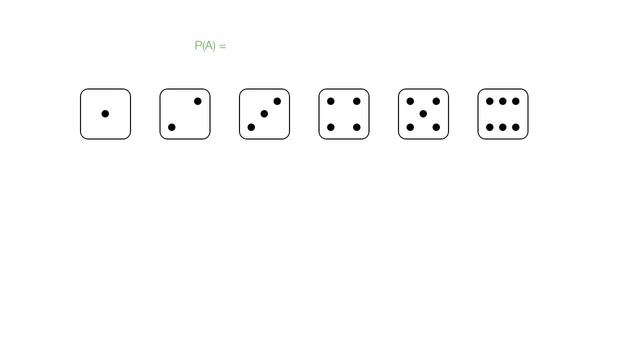 So I have six over six or one, which means everything's covered. Event A is rolling a dice and its value is an odd number, So in this case the die could be a one, a three or a five. There's a one out of six chance for a one, a one out of six chance for a three. 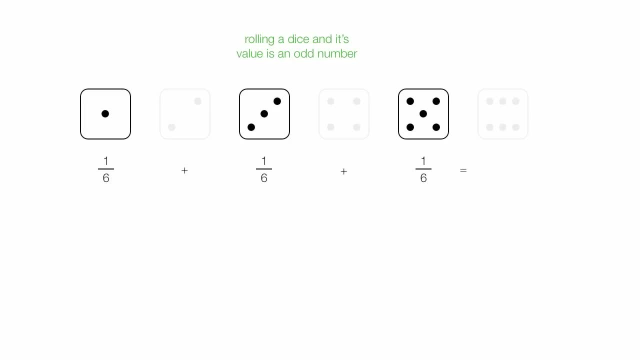 and a one out of six chance for a five. All those ones added up equal to three. So there's a three out of six chance of getting one of those, or about one half. Actually one half, not about is one half. 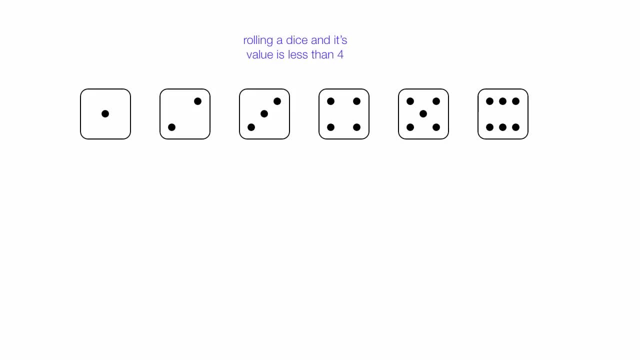 Now Event B is rolling a dice and its value is less than four. It could be a one, a two or a three. There's a one sixth chance for each of these as well, And again, adding these up will equal to three sixths. 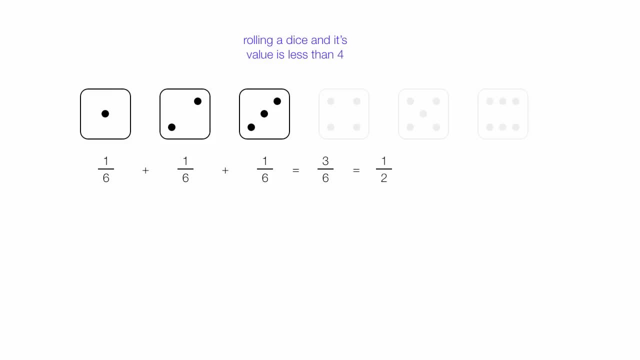 or one sixths Or one half. Let me show this to you also visually, or symbolically as well. Again, Event A is rolling a die and its value is an odd number, So I'll just put in the circle there a one, a three and a five. 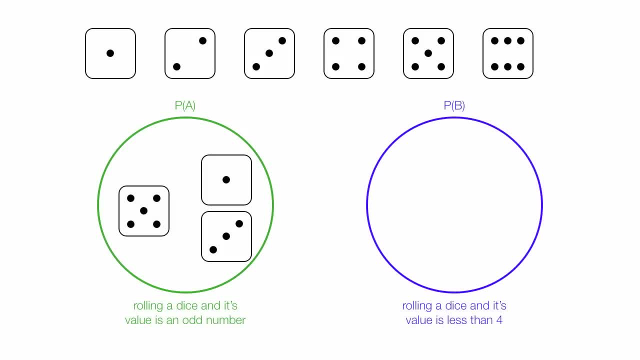 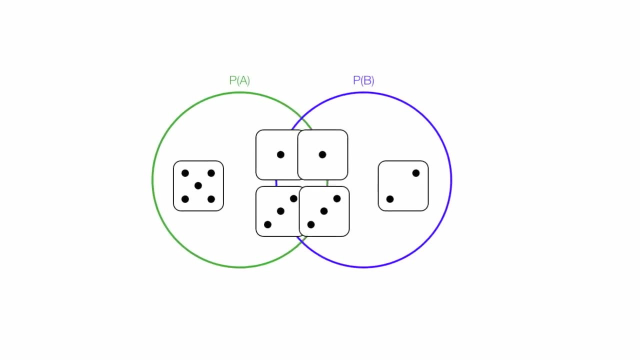 The probability a dice is less than four is Event B, So I'll just put in there one, two And a three Like that. Now, if I take these two events and I find out where they intersect or where they cross or what they have in common, 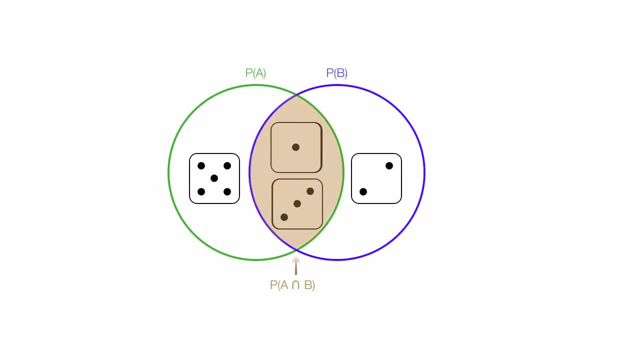 that's the brown area right there, And I write that as the probability of A intersection B, And in this case they intersect two out of six times, or two sixths. That's the probability, Or this equals one third. Again, I'm concerned with the intersection of these two events. 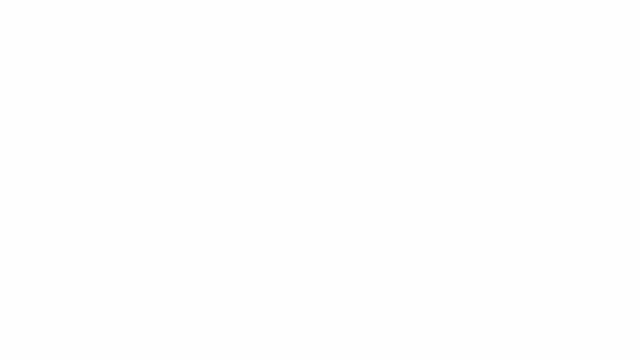 Now I have everything I need to make my calculation. So what is the probability of Event B happening? if I know Event A happened. So again, the P is what is the probability of that's? the P B is rolling a die and its value is less than four. 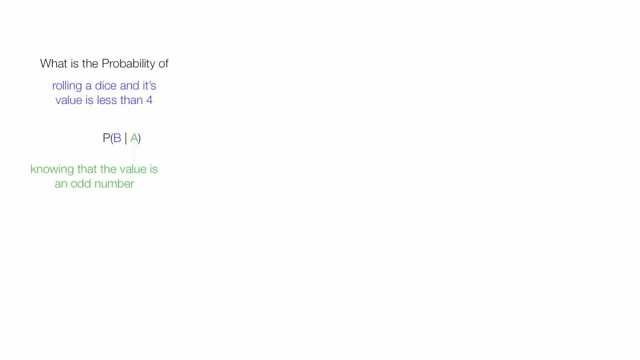 And Event A is knowing the value is an odd number. So this all equals to the probability of an intersection of A and B divided by the probability of Event A, which is equal to one third. Remember, one third is the intersection which we just calculated. 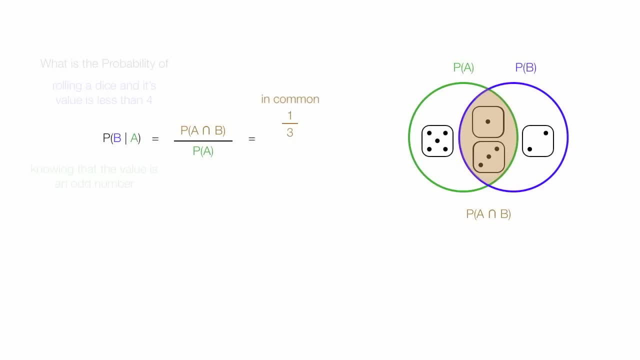 It's what A and B have in common, And that happens two out of six times, And I simplified that to one third And that's where that one third comes from. one over three. And this is divided by the probability of Event A, which is one half. 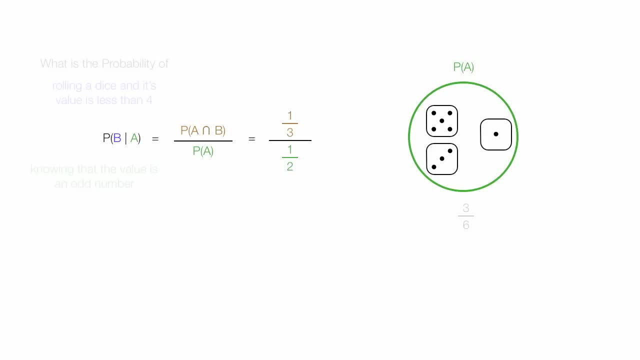 And again, three out of the six possibilities of rolling a die can be an odd number And this simplifies to one half, And that's where the one half comes from. And this equation can be rewritten and simplified as two divided by three or two thirds. 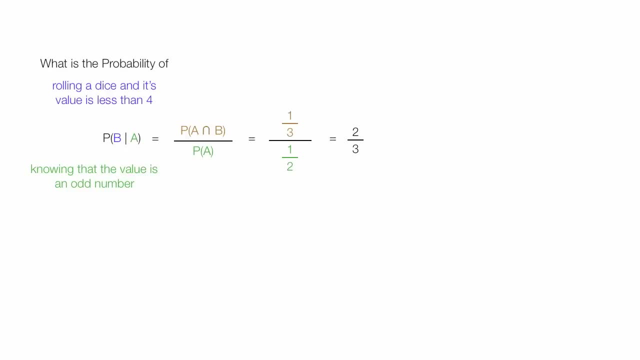 And now here's what this says. It says that if I know that the value is an odd number, two out of three times the dice is going to be less than four. I'm going to change the problem slightly And I'll repeat it. repeat the process, how I solve it. 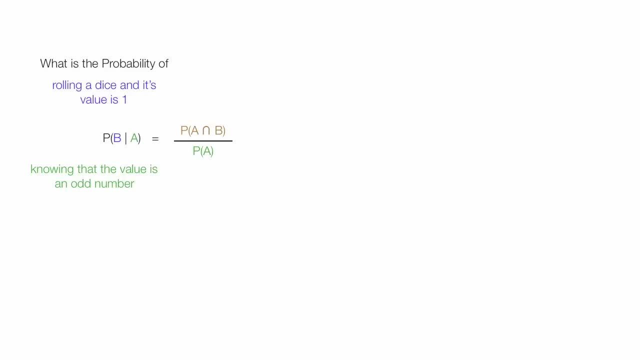 Now, if I know that the value is an odd number, what's the probability that the value is one? The probability of Event A is exactly as it was before, and it's still one half, And I'll go ahead and put that in there. 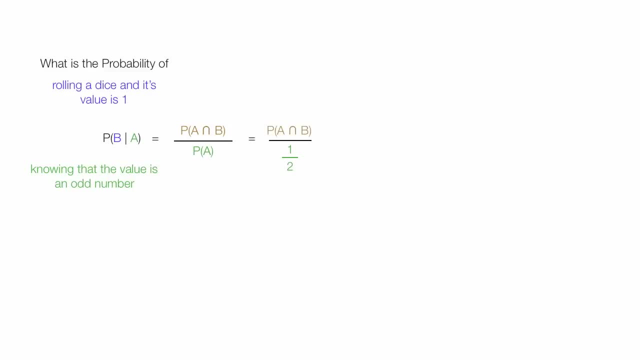 Event B has changed, though, And let me start over at the very beginning, like I did last time. What is the probability of rolling a dice, and its value is one? It's just that blue right there, Or one sixth of the time, one out of six. 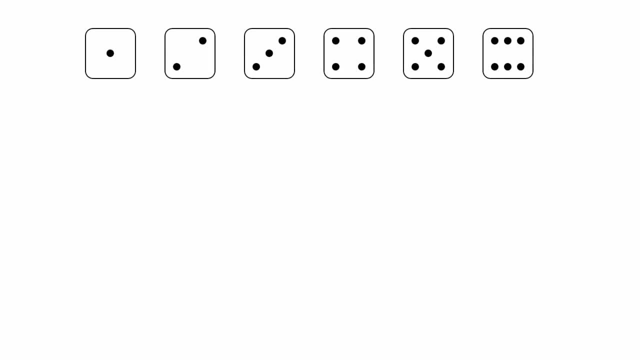 So now I can rewrite this a little visually for you. Probability of A Event A- an odd number is exactly the same as it was last time. The probability of Event B rolling a dice and its value is one, It's just one. 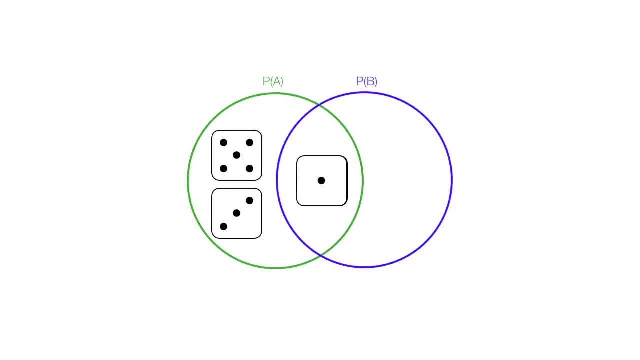 There's only one thing in there: The intersection. now the brown area- becomes the intersection becomes one divided by six, And I'll plug that into the equation. So this all simplifies to one third. In the end this says that if I know that the value is an odd number of a dice that's been rolled, 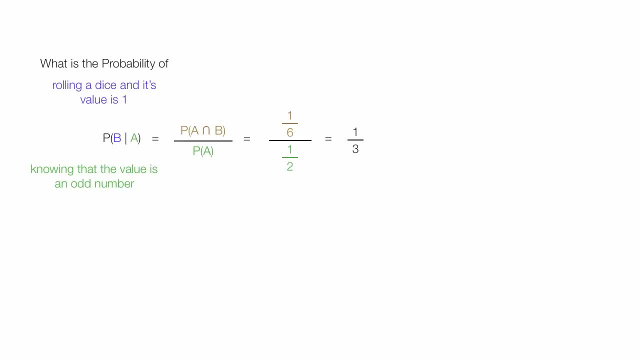 the probability that it's a one is one out of three chance. Hopefully you'll share the knowledge and maybe even like us on Facebook Comments, questions and requests below, And don't forget to subscribe because I'm always posting new material. to help you in your stats class.